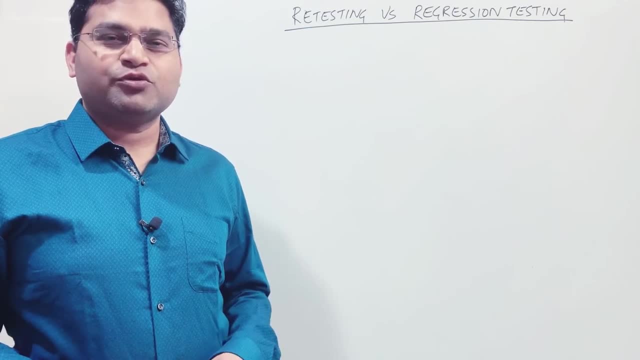 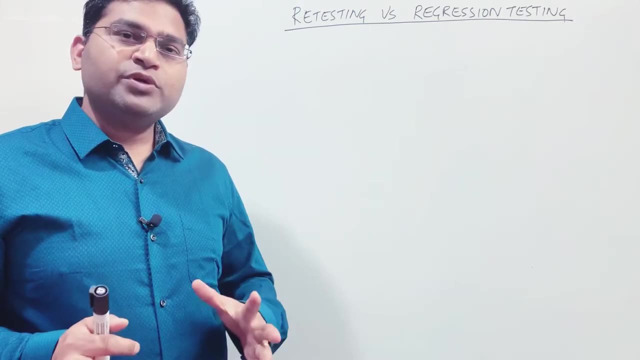 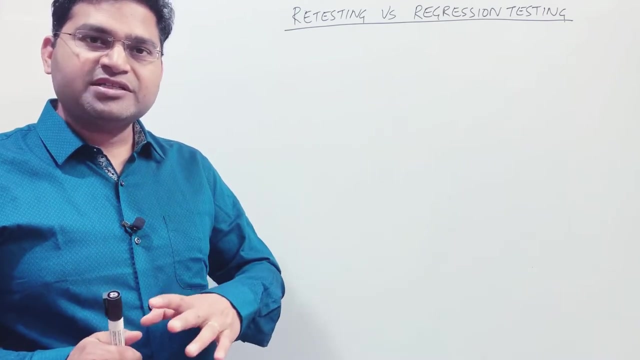 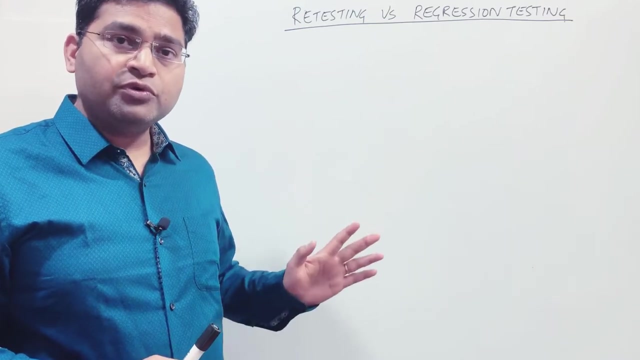 Hello everyone, welcome again. In this software testing tutorial we are going to understand the differences between retesting and regression testing. So before we get into the differences, first let us understand what is retesting and regression testing. So regression testing I have already explained in detail in previous two tutorials. So if you haven't watched those two tutorials, please watch them through and then come to this particular tutorial, because in this one I'll explain what is retesting and what is regression testing. 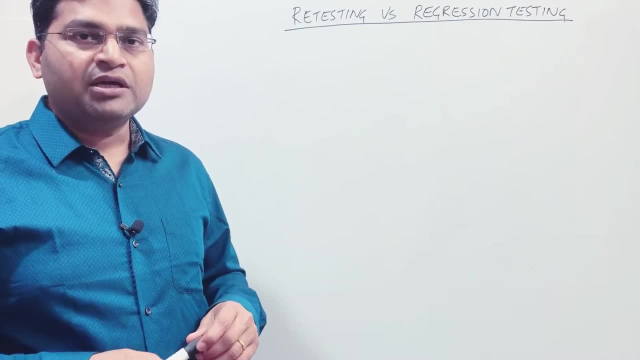 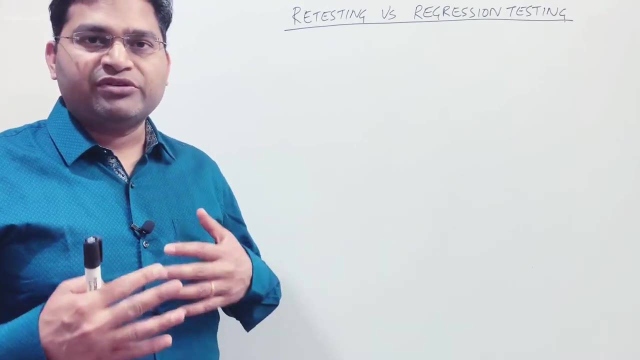 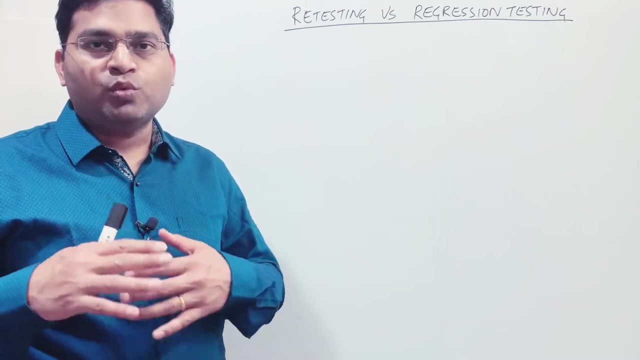 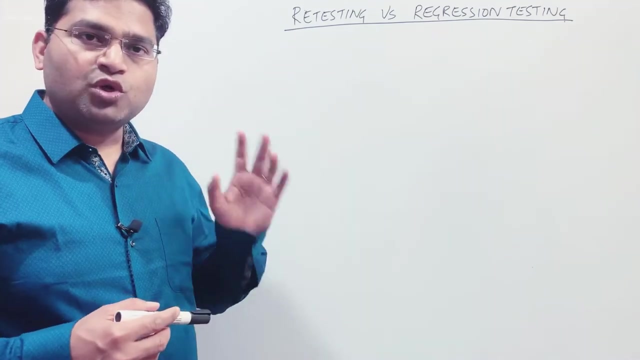 And then differences between retesting and regression testing. All right, So this is very important interview question. So you need to understand, with example, how you will be able to explain differences between retesting and regression testing. And also, when you're working in any project, you will be very much requiring when to use the term regression testing and when to use retesting. All right, So before So let's first understand what exactly is retesting. I'll start with an example, because unless until you know the example, you won't be able to understand. 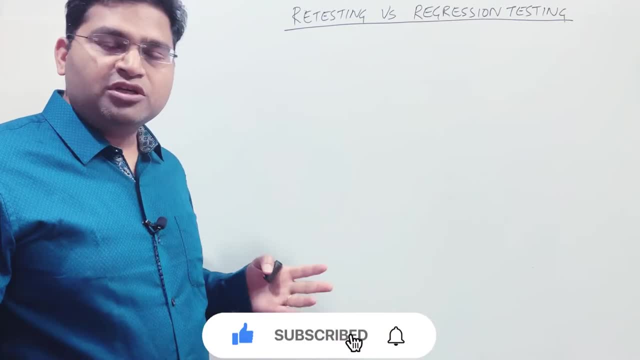 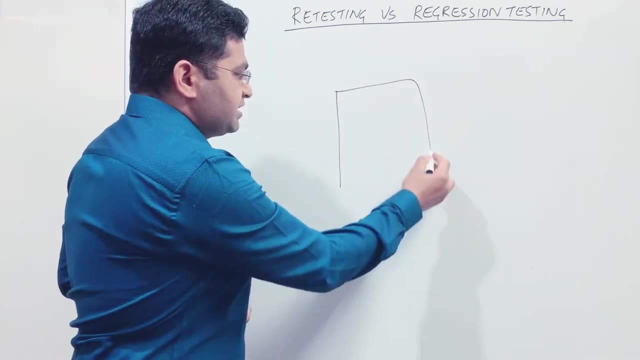 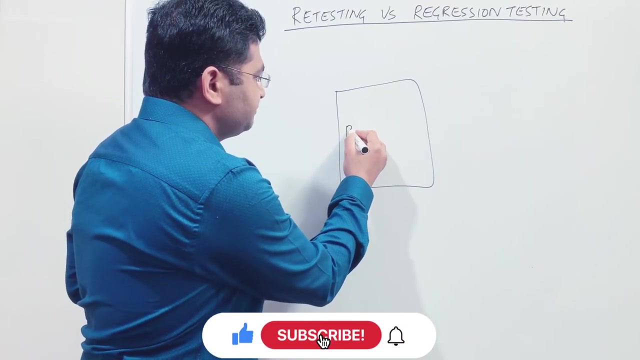 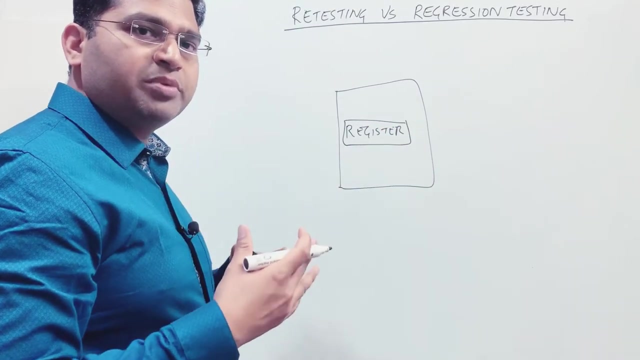 You won't be able to explain it properly, Right, So I'll take an e-commerce example that we have been taking throughout this tutorial series. So I'll take a login or registration example. All right, So in the e-commerce website, we have the registration functionality. So say, for example, I have a register functionality, Okay, And this register functionality could be with the use of email, with the social media account, for example, Facebook, Twitter. 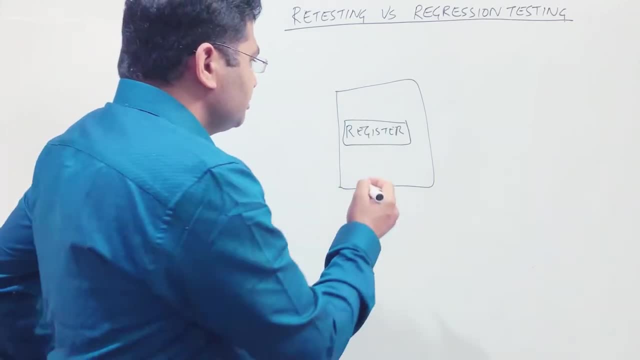 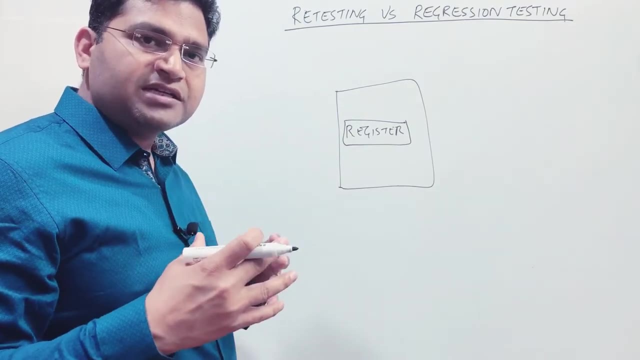 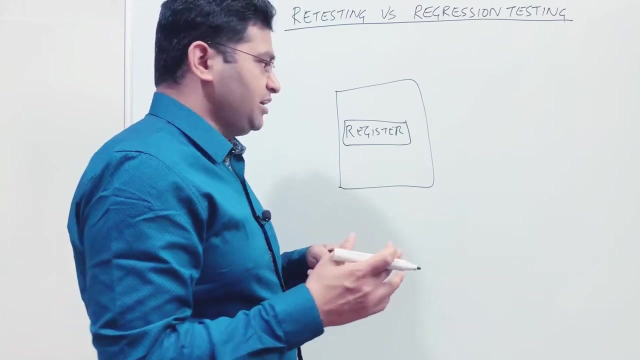 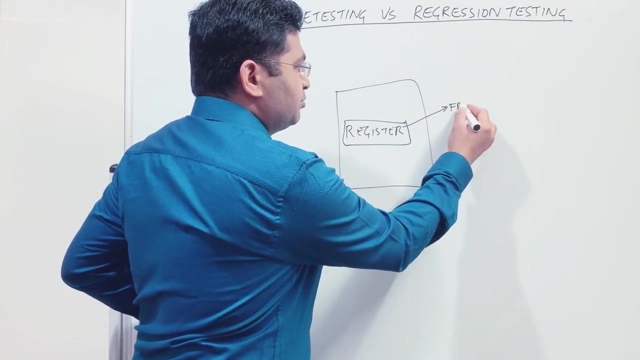 And you know Google account as well. So say, for example, now register functionality is one functionality And then there will be, you know, smaller modules within this functionality to basically cater for registration using different social media accounts and the email address. Okay, So say, for example, register has the functionality or the capability to register using Facebook account, using Google account- Right, 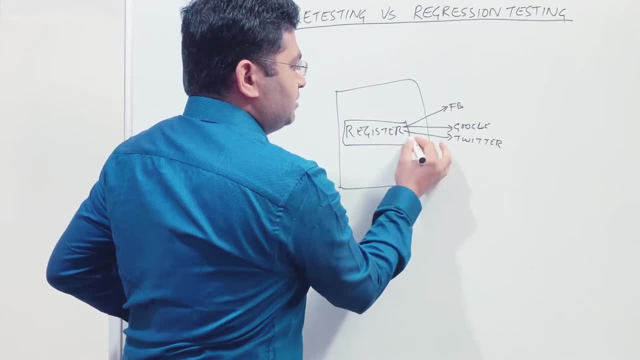 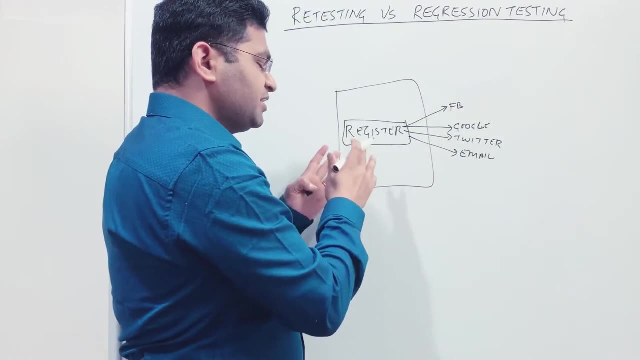 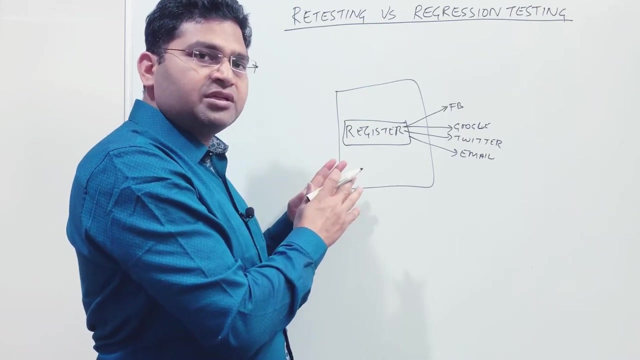 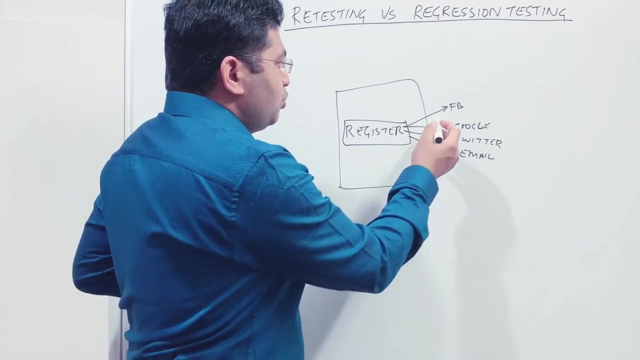 Using Twitter and using email, Say, for example, as part of your project, you have the register functionality. You have to build an e-commerce portal And in the e-commerce portal you have to provide the functionality of registration. with these four, you know different types of registration capabilities in the e-commerce website. So when you, as a testing team or as a tester, start testing, 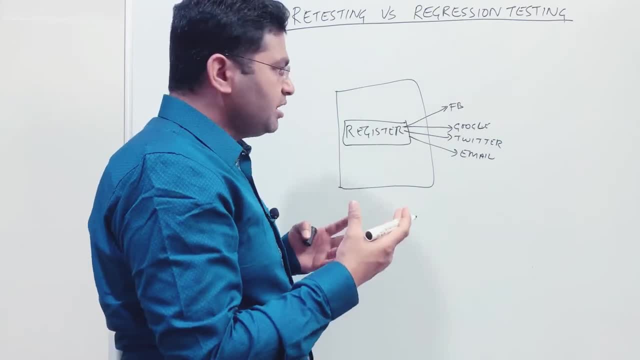 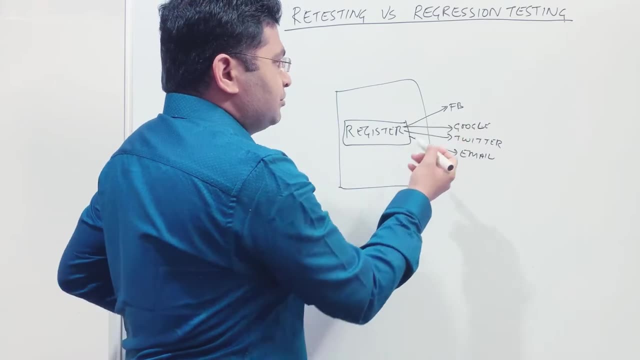 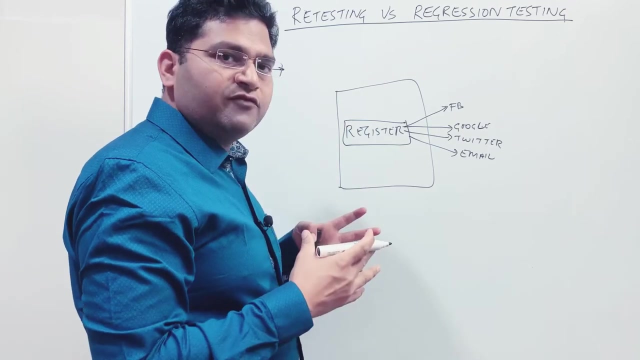 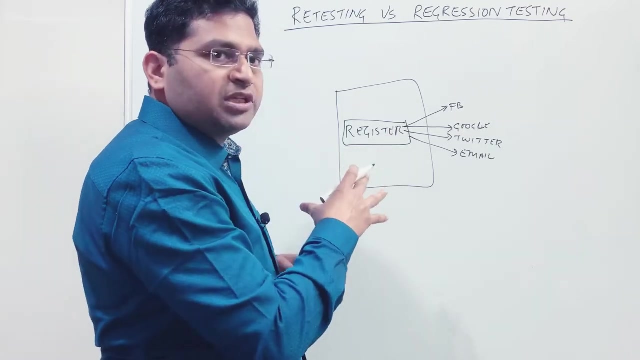 Getting a small build. if you're working in Agile or Scrum, then Agile, Scrum, basically- then you will be getting these features, as you know, say Facebook registration or Google registration. So one at a time you'll be getting these. or if these are small features that need to be developed by the development team, And if they can be developed all together at once, you'll be getting all of them at once. But in terms of testing, you have to basically verify, you know, registration using Google account. 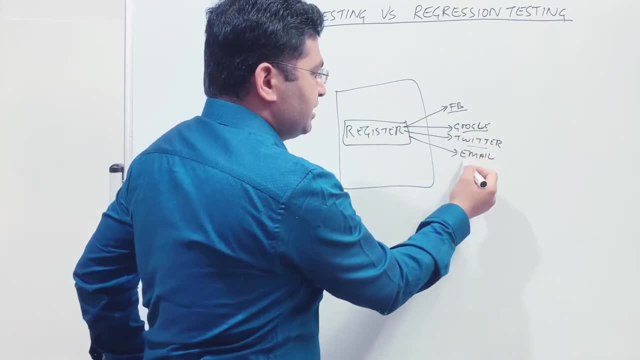 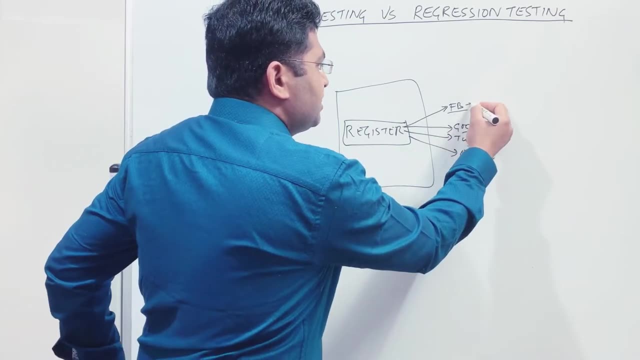 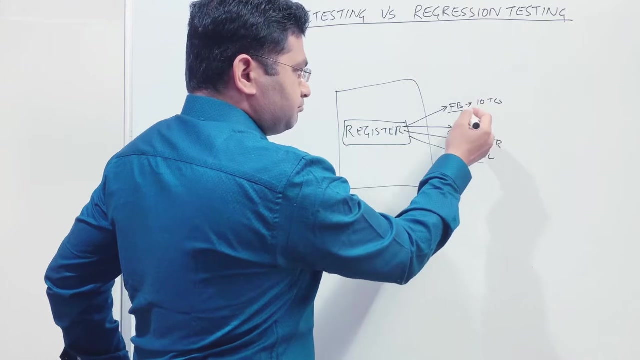 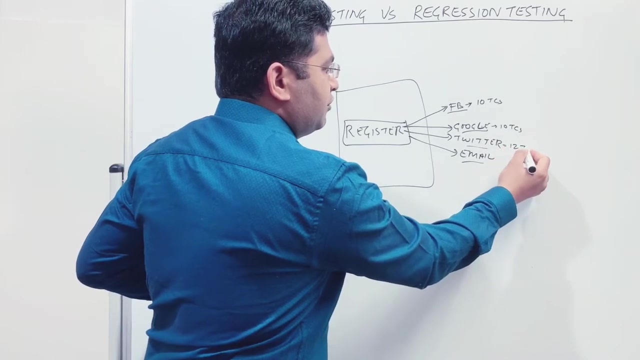 Using Facebook account with Google account, Twitter and email. So you'll be writing some test cases for each of these scenarios, or each of these you know, registration functionalities. Now say, for example, I have written, you or you have written 10 test cases for the Facebook registration functionality And then you know, like, similarly, 10 test cases for Google, 12 for the Twitter. Maybe Twitter has some more additional functionalities that need to be registered. 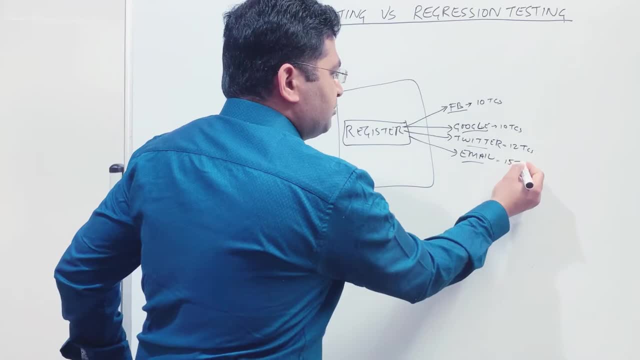 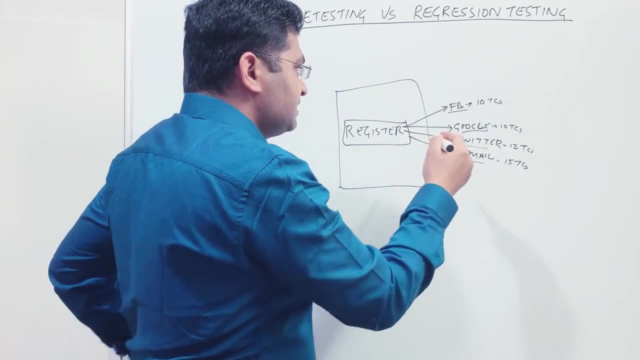 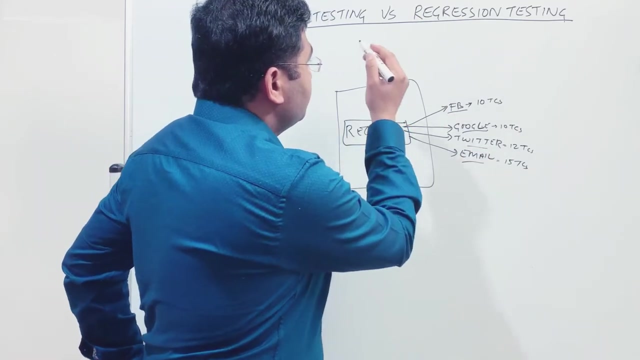 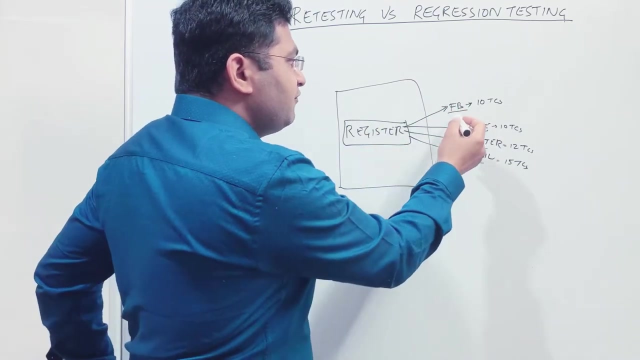 Verified, you have 12 test cases And for email, say, for example, you have 15 test cases written. All right, So all together, these are, you know, the test cases that you need to verify for the register functionality of the e-commerce portal. Okay, Now, when we talk about retesting, basically, so what retesting is? so when you are basically verifying this register functionality and say, for example, when you are testing the Facebook registration and you are executing these 10 test cases, 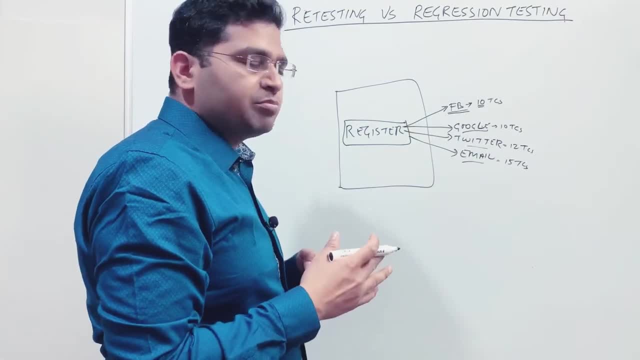 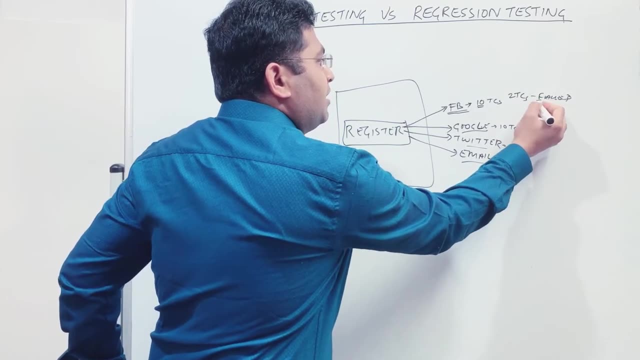 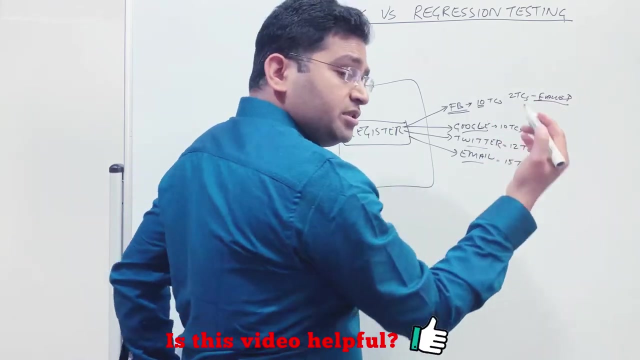 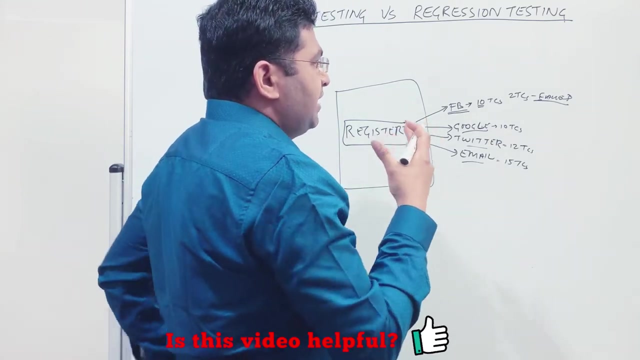 and out of these 10 test cases, eight of them passed, but two of them failed Right. So two test cases failed. Okay, Now these two test cases that got failed, in case you know you. so once the test cases will fail, you will basically raise the defect. So once the defect has been raised for those test cases, those defects will be assigned to developer or development team. 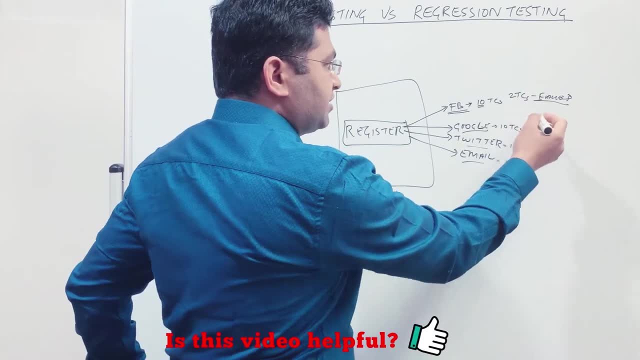 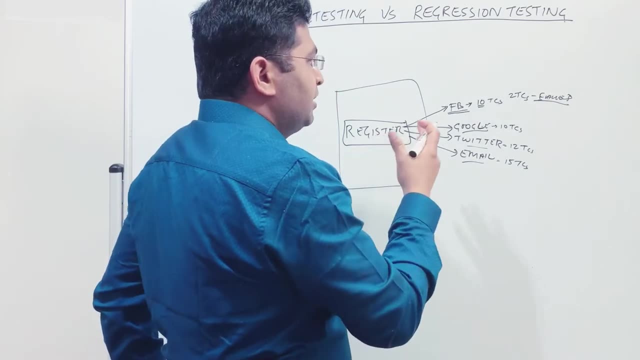 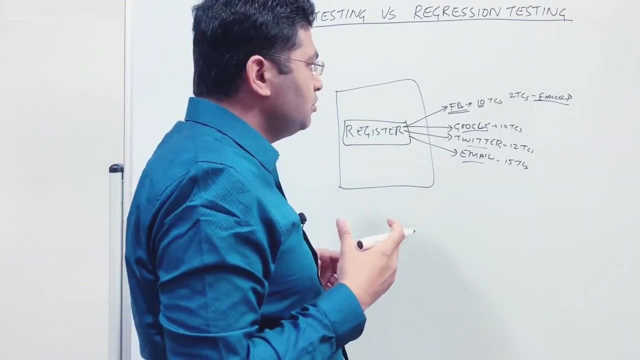 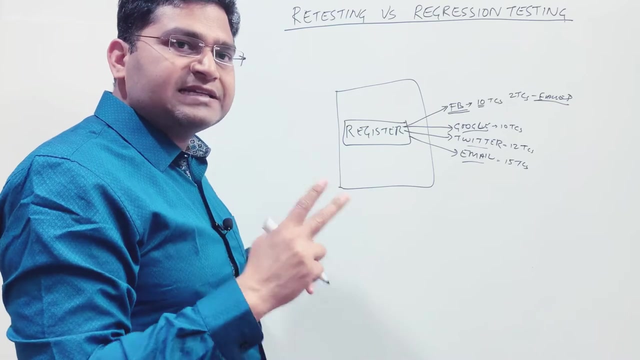 And developer will work and fix those defects Right. So now, when these defect fixes are available to you and deployed, then you will be verifying or you will be retesting, basically those two test cases. Right, So you will be verifying those two defects And if you are just executing those two failed test cases that failed out of these 10 test cases, then that is known as retesting Right. 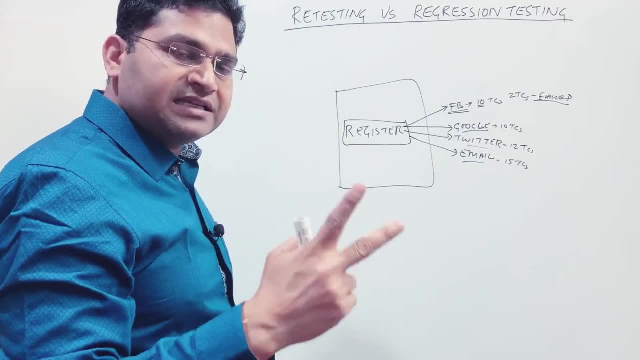 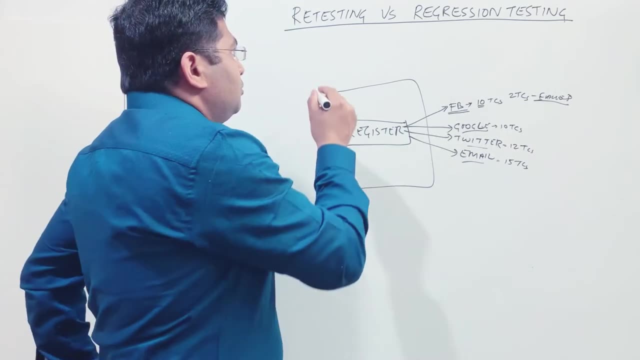 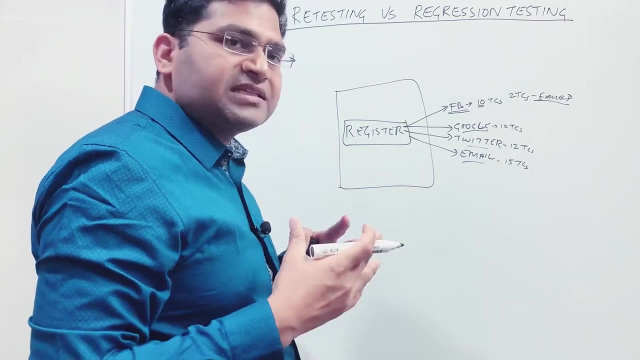 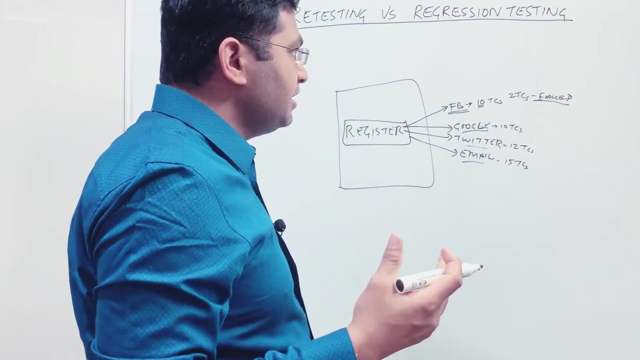 So you are just executing those two failed test cases and verifying whether now those two test cases are getting passed Right? So when we talk about retesting, retesting is basically executing the failed test cases or any test cases again. So same test cases which you want to execute or retest. that is known as retesting. Okay, Now if we talk about regression testing, so we'll take the same example. 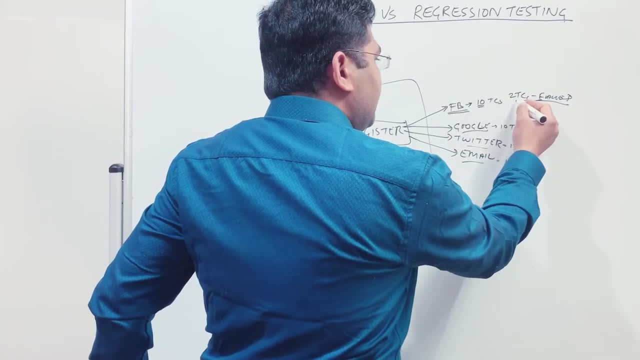 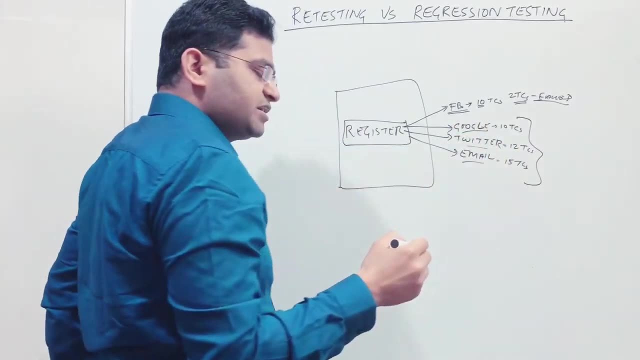 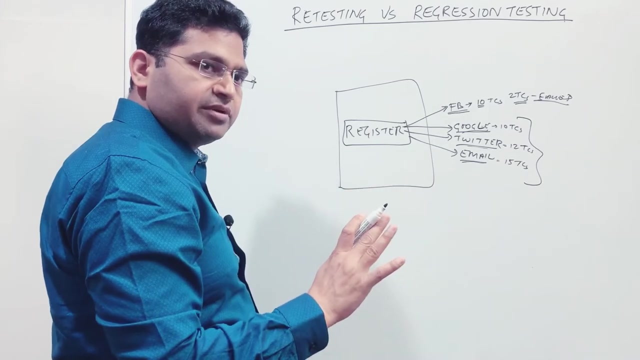 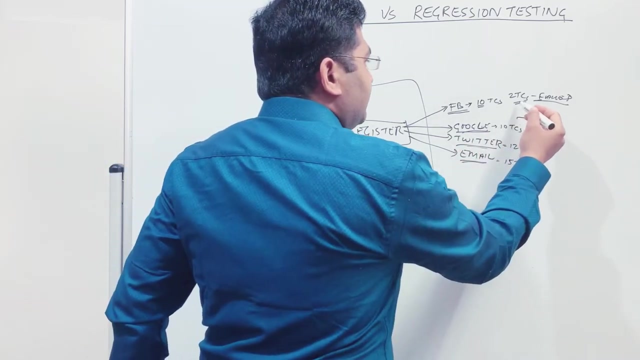 For example, this FB registration got failed and two of the test cases got failed and you have raised the defect. but all the rest- registration functionality has passed. So Google registration, Twitter registration, email registration, all of the test cases have passed Right Now. when we say regression testing of this particular feature, what you do is you don't not only re-execute the two failed test cases, but you also analyze any code that is not working. which is the one that is not working Right? So you will be verifying those two failed test cases, Right? And then you have to go back and run some testing, Right. So these tests that failed are not the ones that are lasting for a long period of time. In fact, it's the ones that are lasting the longest, Right. So if you click here and you click on the test test, you can see that it is still working. For example, this FB registration got failed And two of the test cases got failed and you have raised the defect. But all the rest. 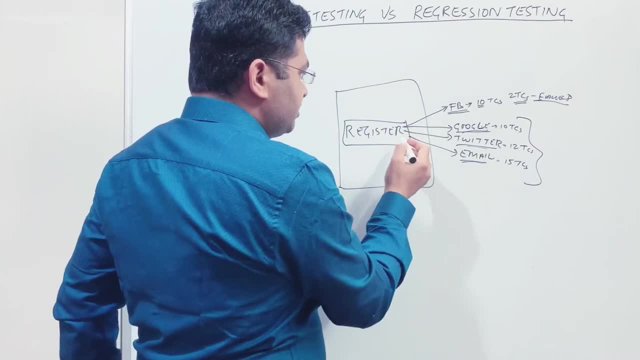 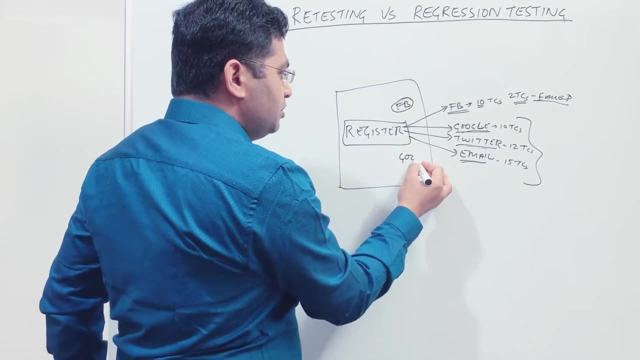 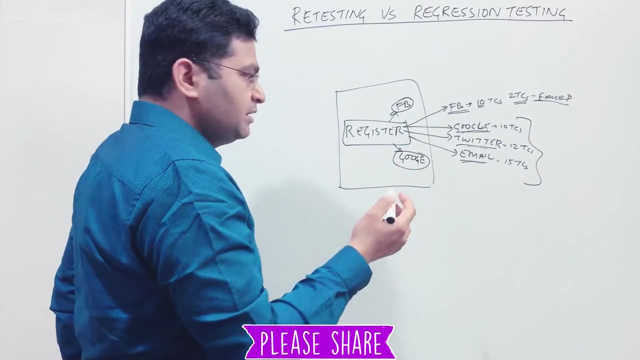 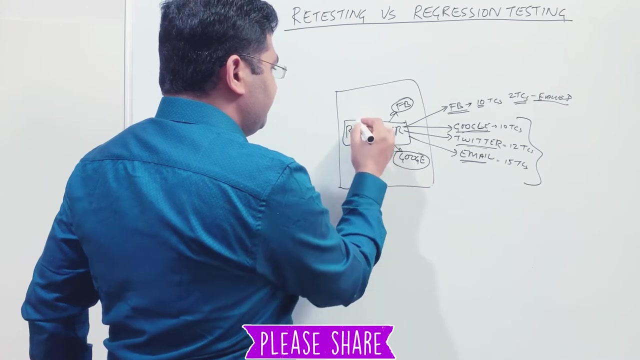 of the surrounding features. so, if we talk about registration, we have fb, right, so there is a registration using fb. there is a registration using google, right? so for which you have test cases. so these are all related modules of the registration functionality, right? so you have twitter and we have email, all right, so these all are related modules of the registration. 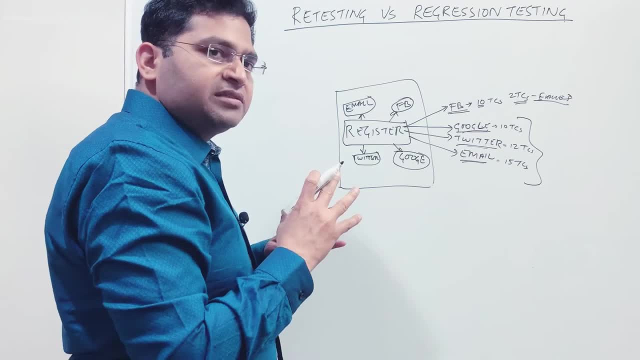 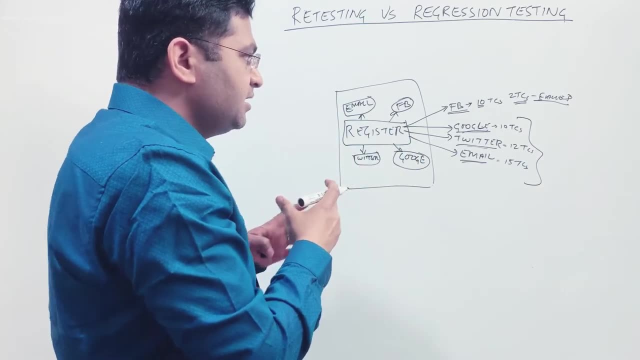 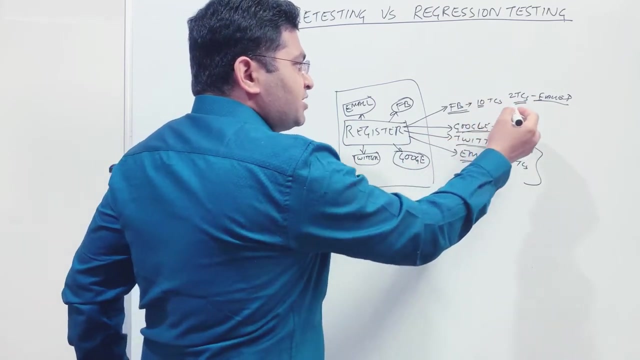 functionality. now, when you analyze all the related modules of a particular functionality and you come up with the test cases that need to be executed because they are related to the those failed test cases- say, for example, because of these two failed test cases, you also want to verify that Google registration, Twitter registration and email registration. 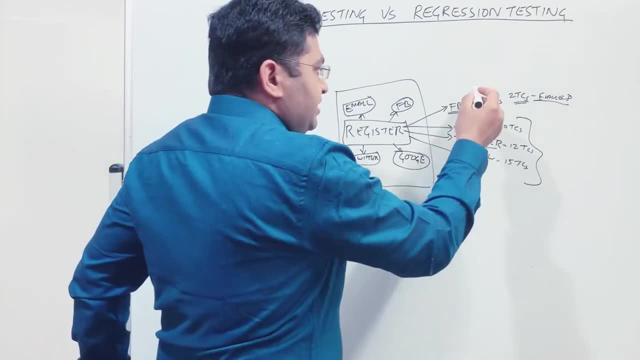 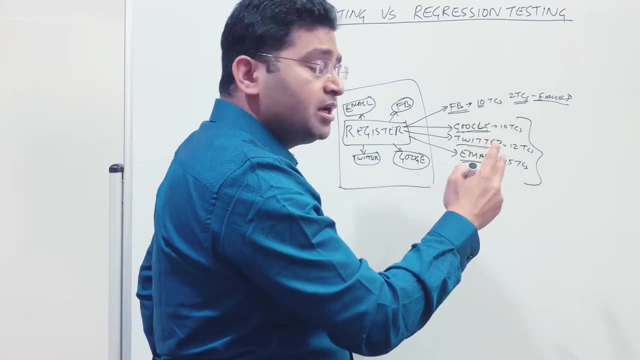 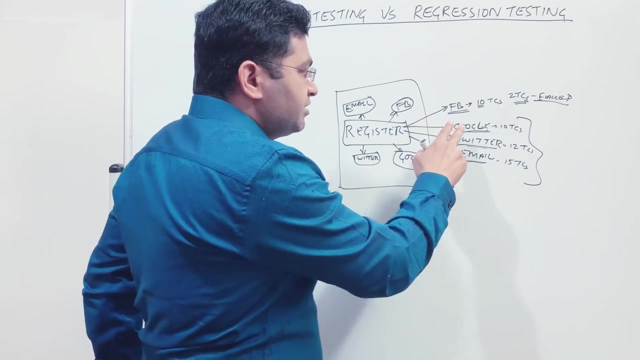 hasn't been impacted at all. right, Because in the first round of execution everything was passing- Google, Twitter, email and Facebook- only two test cases were failing. But when you got the fix for those two defects, you also want to ensure that the existing functionality or the 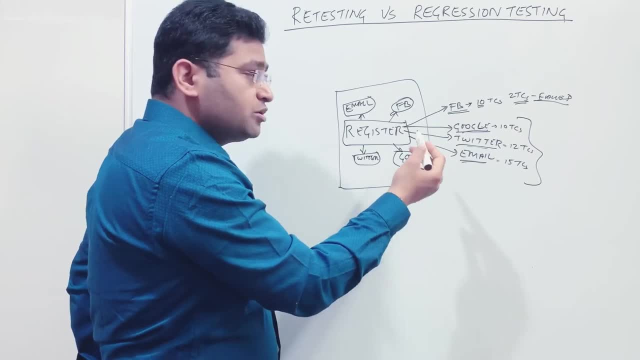 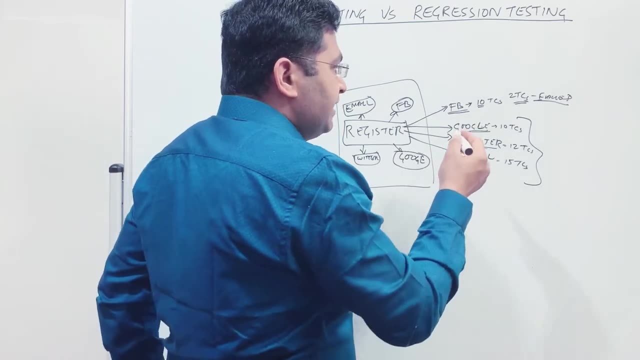 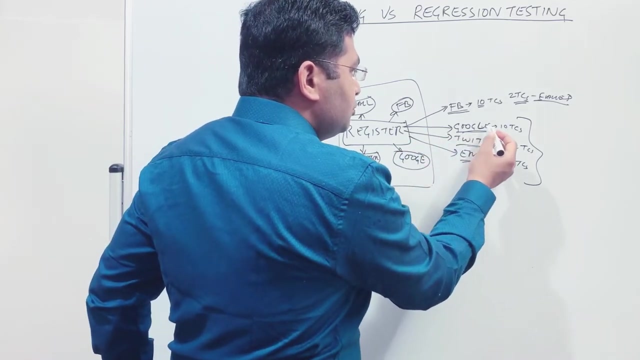 existing registration that was passing for Google, Twitter and email. it still passes, right. So that analysis- and if you want to execute or ensure that those test cases are working perfectly fine, then in that case what you do is you either re-execute all of those which are related or 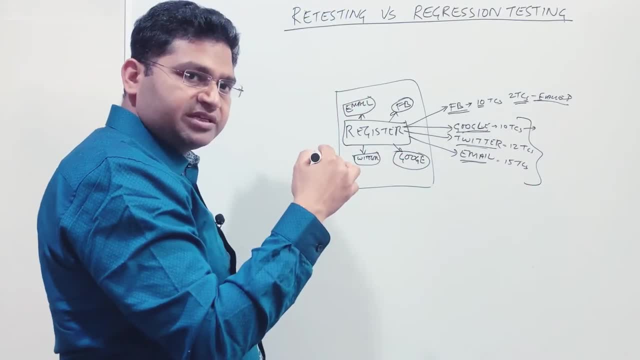 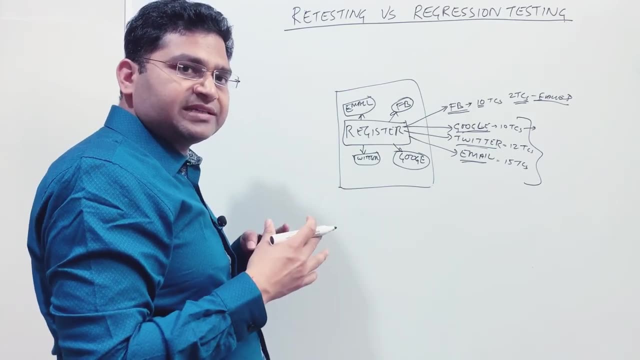 you basically pick the critical ones right. So, which I have explained in the regression tutorials already- What are the different techniques, how you will analyze the regression test cases that need to be executed. So here, in this particular case, say, for example, two test cases were failed and I want to re-execute. 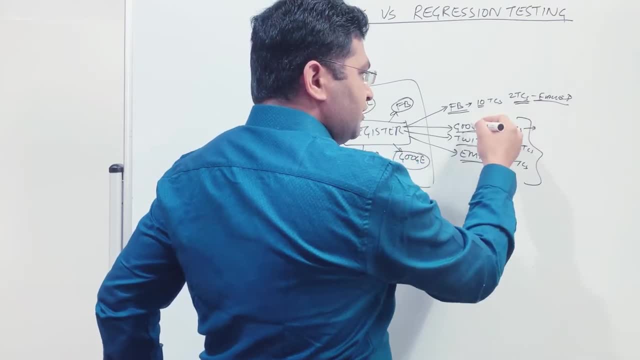 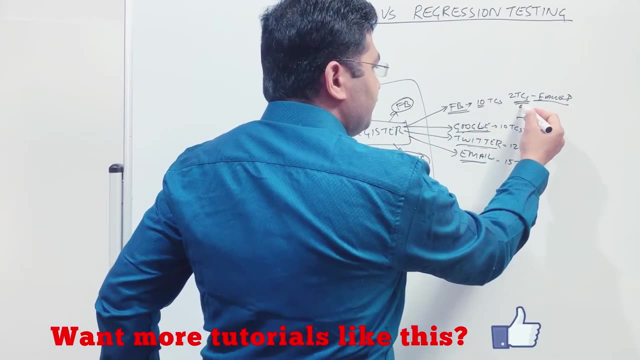 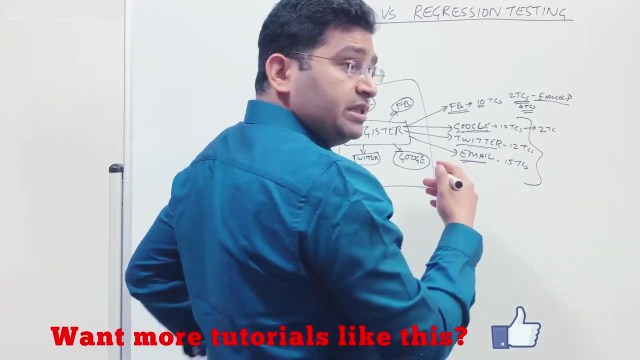 for the Facebook. So I like to say I'll pick two test cases for the Facebook that got failed and I'll pick, you know, a couple of other critical test cases. So say, for example, four test cases I want to execute in the Facebook functionality two test cases for Google, just to ensure that Google